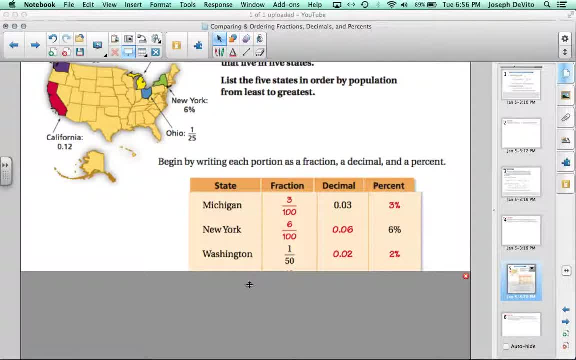 into decimals or percents, Because the numerator at that point is the one that's always going to be in the denominator, and the denominator in the denominator is the one that's always. that point is the percent value. so two one hundredths is the same as one. 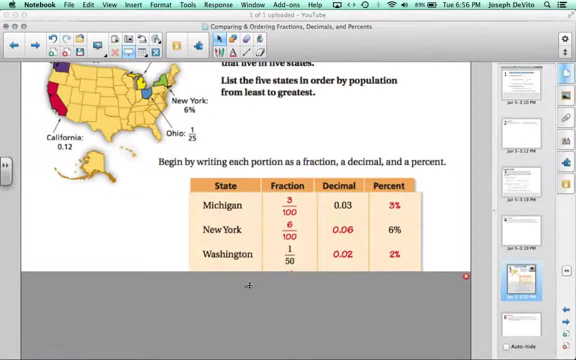 fiftieths. so we get two percent and zero point zero two, and California was given as zero point one two. we move the decimal point twice to the right to give us twelve percent, and of course twelve percent is the same as 12 out of 100. and 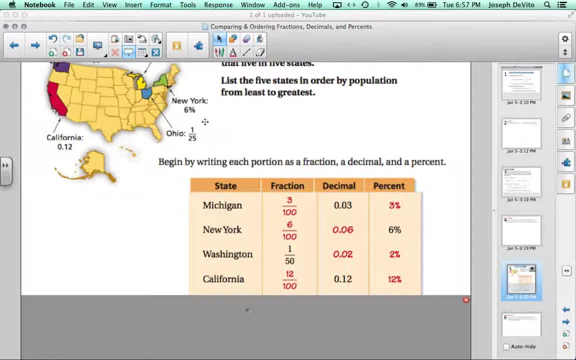 lastly, Ohio, 125th. think about what you would have to do here to convert this into a percentage. all right, of course we would look at 25 and say, hey, that's four times less than 100. so if we multiply 25 by 4, multiply 1 by 4, we will. 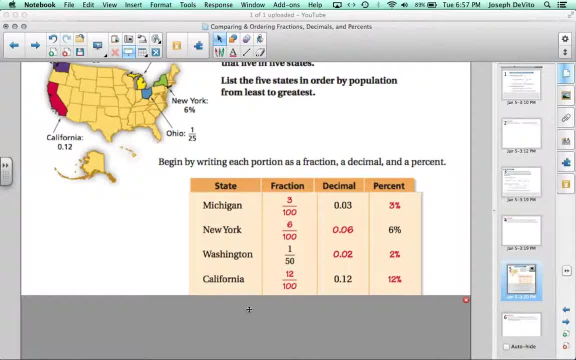 get you know, we'll be able to move into decimal and percentage form. of course. when you do that, you get four one hundredths. so four one hundred says a percent is here and as a decimal is here. so where do we go from? here we are again. 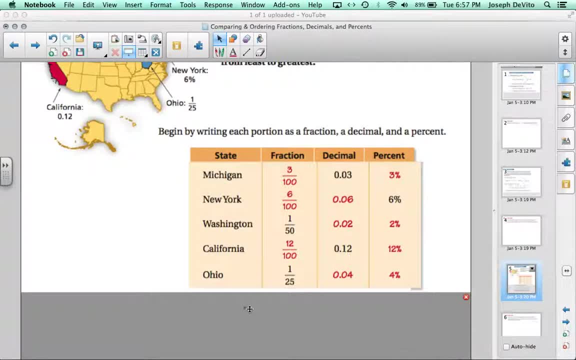 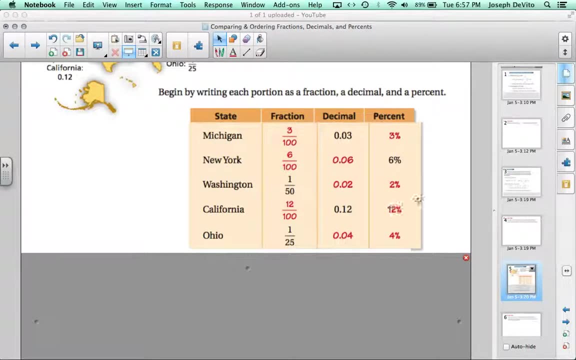 being asked to list from link to the next slide to greatest, and so think about for a second what those would look like. how would you compare these? what's the best way? you could use the percent form, or you could use decimal form and list them from least to greatest. so think about. 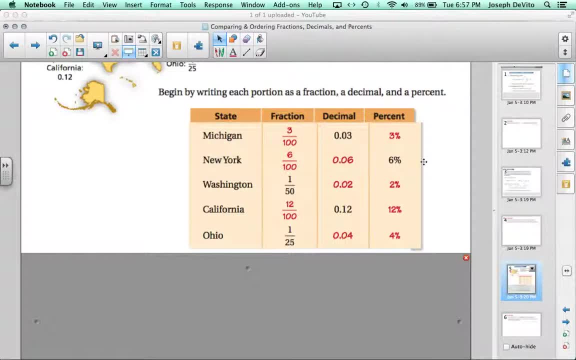 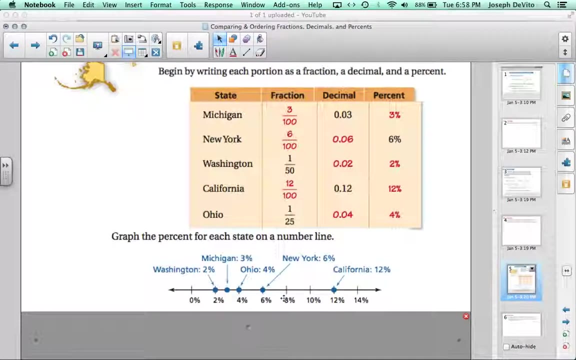 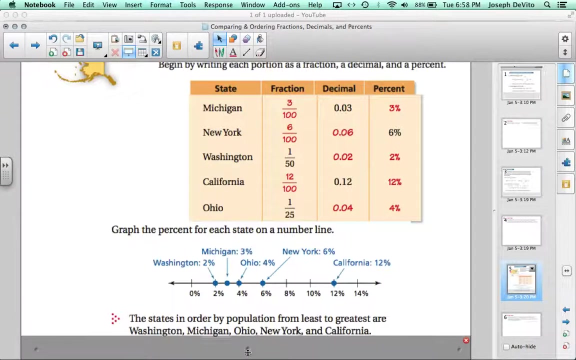 how you would list these from least to greatest. for a second, and let's see if this number line matches up to what you are thinking, you can see all the values from least to greatest on the number line and here they are written out: Washington, Michigan, Ohio, New York and California. those are the populations in 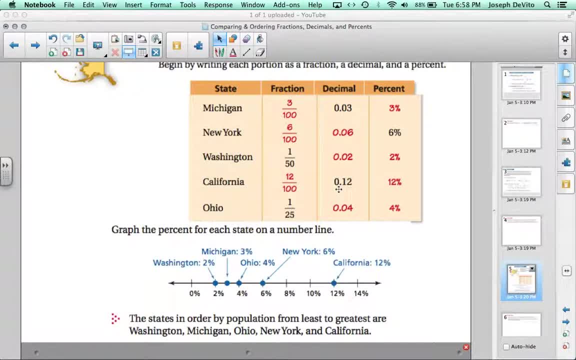 order from least to greatest: V: 0 to the percent sign Apostle ование and m Necron genes.